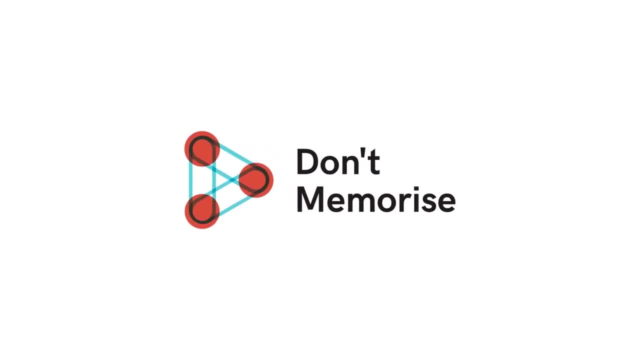 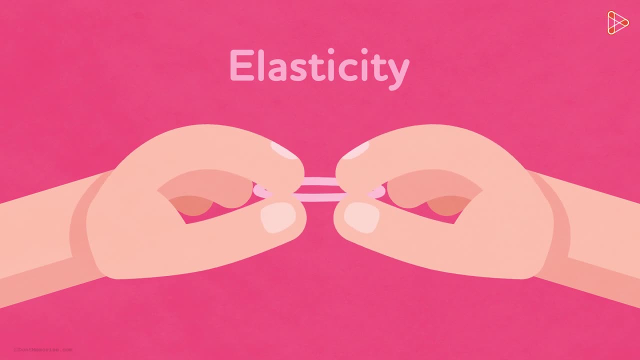 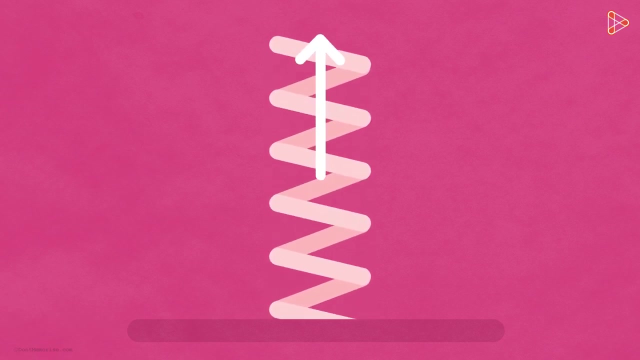 When we hear the word elasticity, the first picture that comes to our mind is something like this: But is this really what elastic means? We will find that out in this video. Let's take an example of a helical spring. When a force of compression or tension is applied, the helical spring gets deformed. 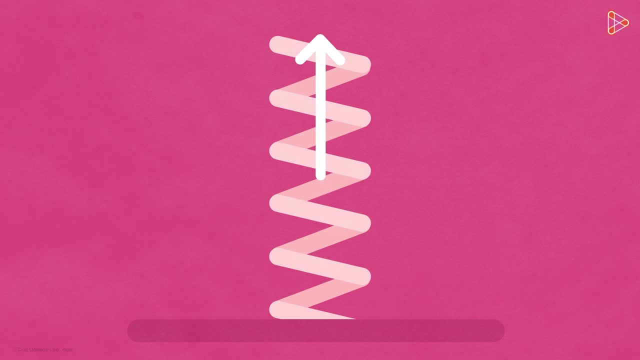 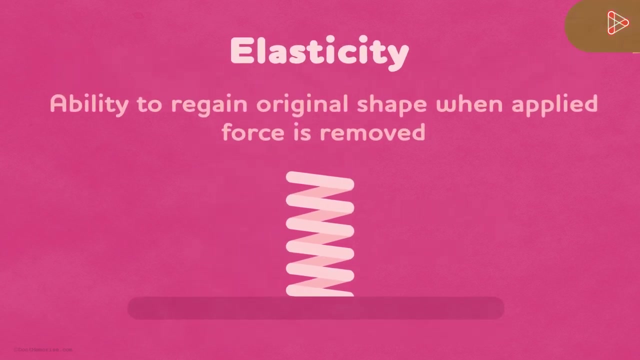 ie it changes in shape or size. This force is referred to as the deforming force, And the ability of an object to regain its original shape when the influence of this deforming force is removed is called elasticity. More examples of such objects include sponge balls and rubber bands. 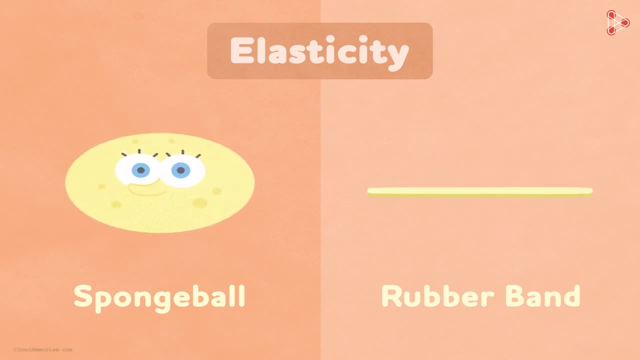 When compressed or stretched, they get deformed, but they soon return to their original shapes. This self-reversing deformity the object goes through when force is applied and removed is called elastic deformation. But is there a limit to the elasticity of an object? 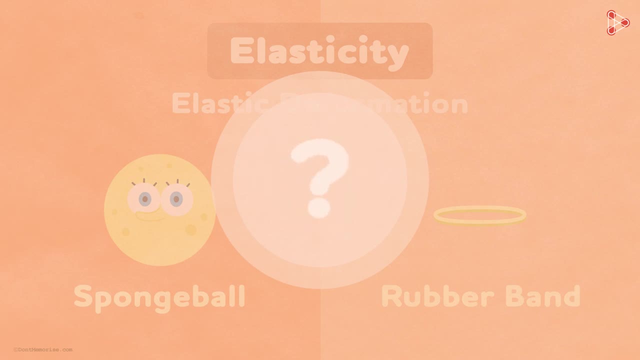 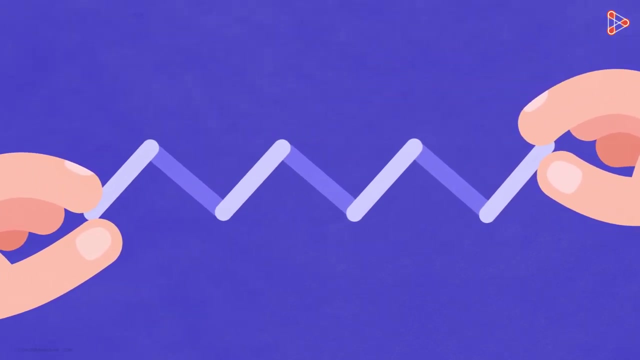 Do elastic objects remain elastic forever? Not really. For instance, if a great amount of force is applied to a spring, it simply won't be able to stretch further than a certain point. But if the force becomes excessive, the spring will get permanent. 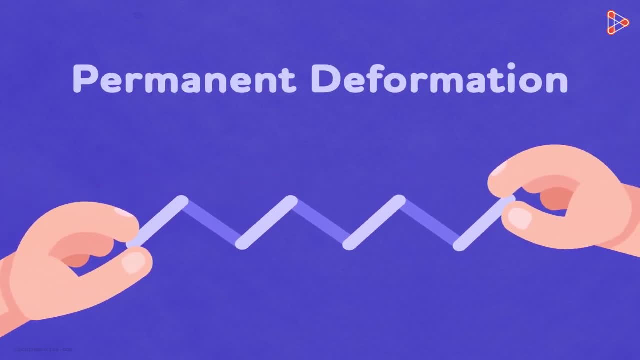 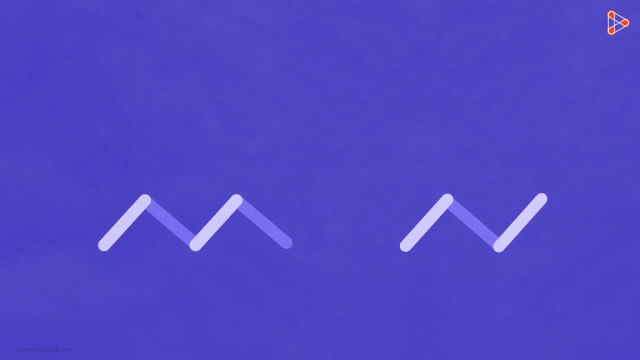 So if the force is applied to a spring, it simply won't be able to stretch further than a certain point. The spring will be permanently deformed and may even break if we keep increasing the force. Hence the spring does not remain elastic forever. 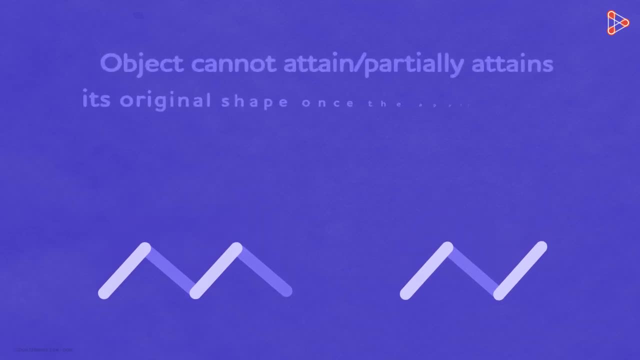 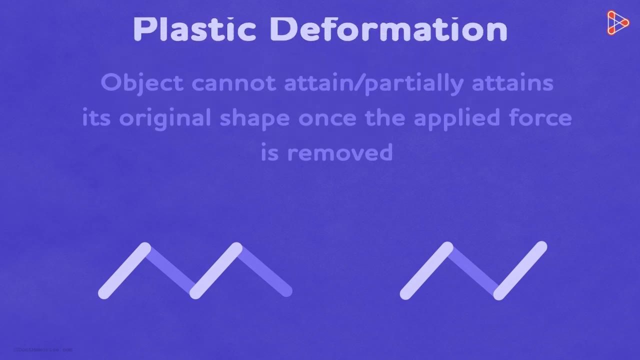 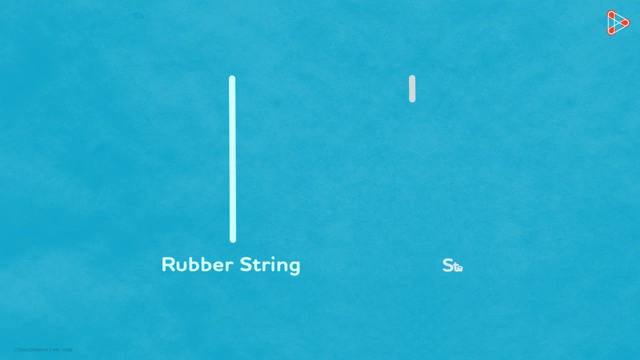 This type of deformation, where the object is unable to attain, or if it only partially attains its original shape once the deforming force is removed, is called plastic deformation. Now let me ask you a question. Suppose we have a rubber string and a string made of steel. 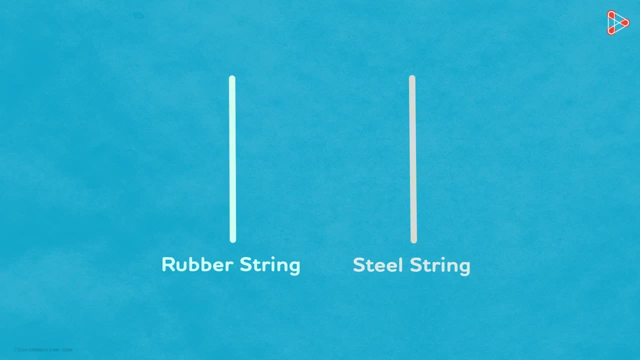 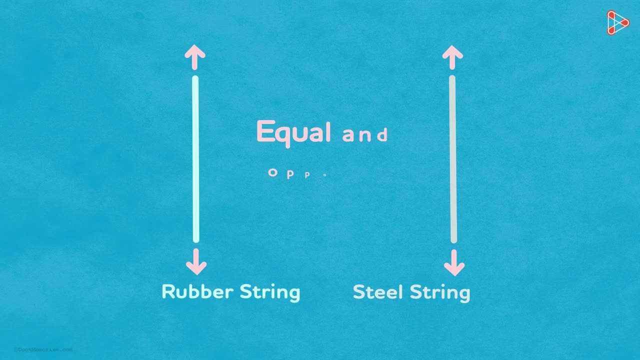 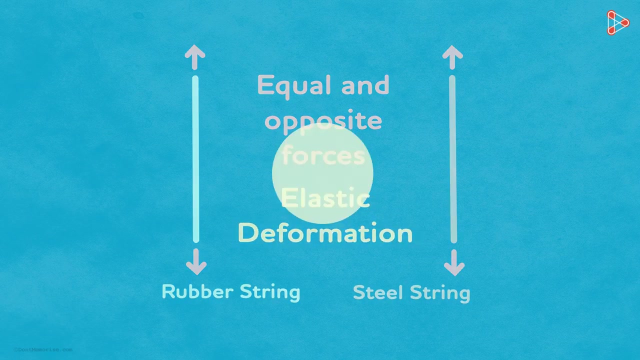 Both are very tiny thicknesses. Both are identical to each other in terms of size and shape. If we stretch them from both the ends with equal and opposite forces, then which one will stretch the farthest, assuming the deformation is elastic in both the cases? 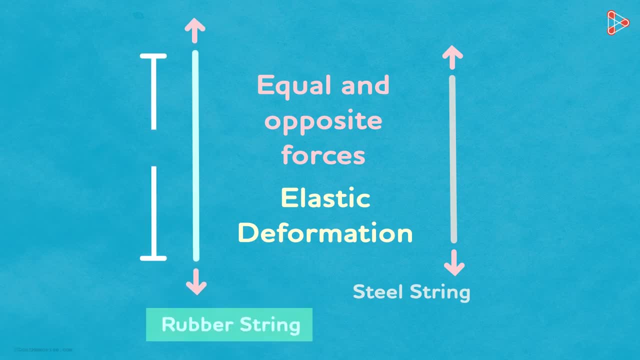 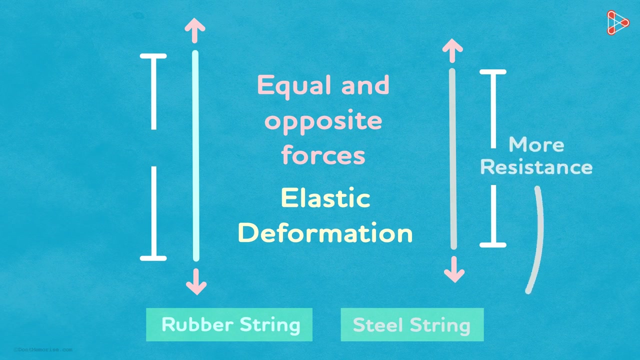 Quite obviously the rubber string will stretch the farthest. The steel string would barely stretch, but it is important to note that it would indeed stretch no matter how little. It doesn't stretch as far as the rubber string because steel applies more resistance to the